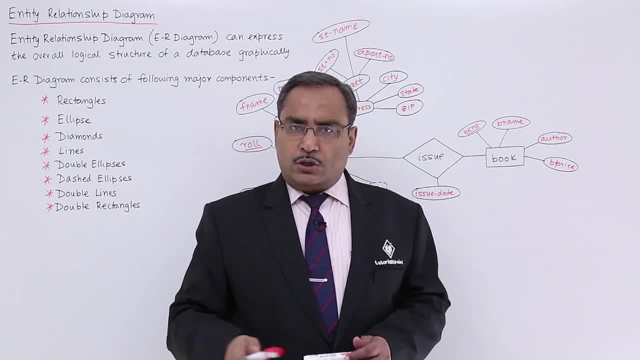 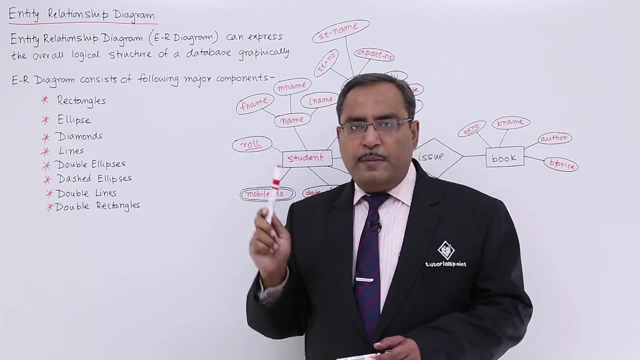 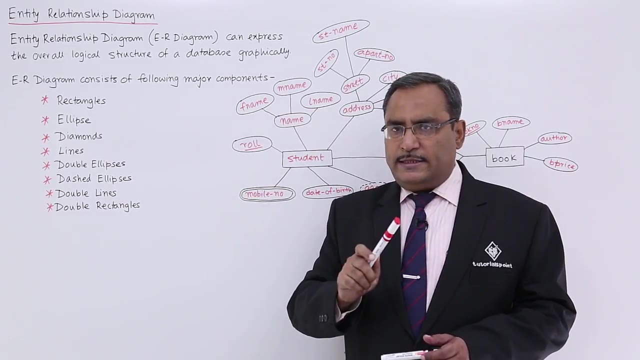 role to represent one database. So here is the definition, which we have discussed already. This ER diagram consists of the following major components. First one is the rectangle. Rectangles will be denoting entities, So entities will be enclosed within rectangles. 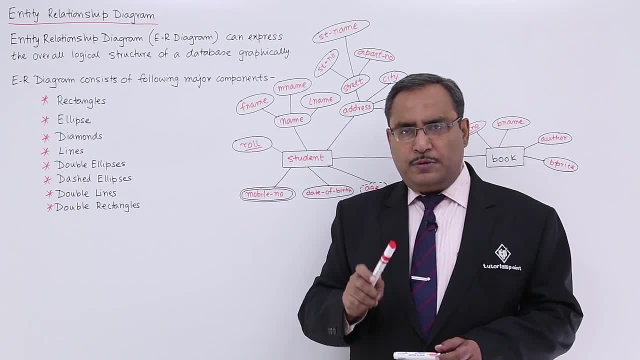 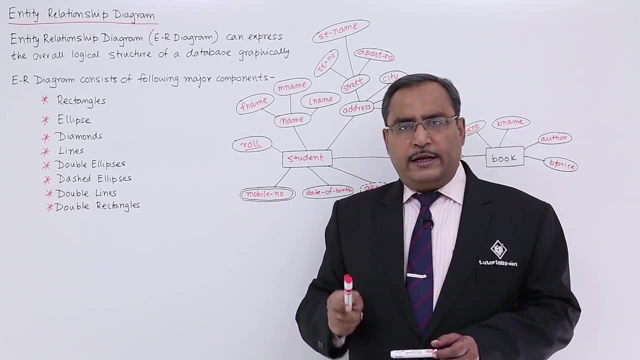 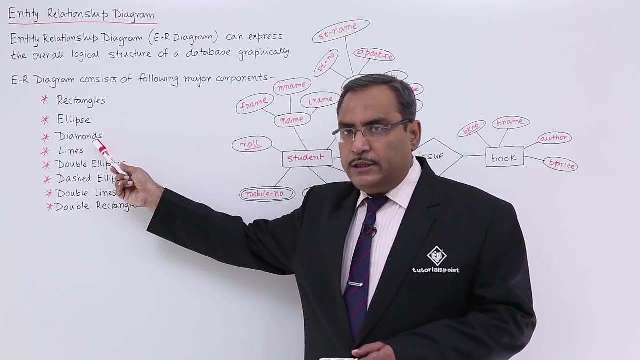 Ellipse will be denoting the attribute, So each and every attribute must be enclosed within ellipse. Diamonds will be denoting the relationship. What is the relationship? What is entity? What is attribute? We have discussed everything in our prior videos. Diamonds will be denoting the relationship. 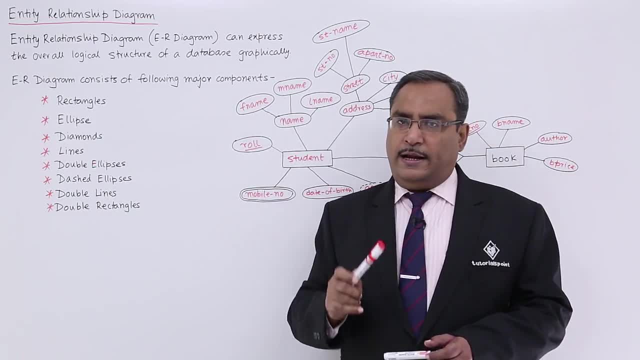 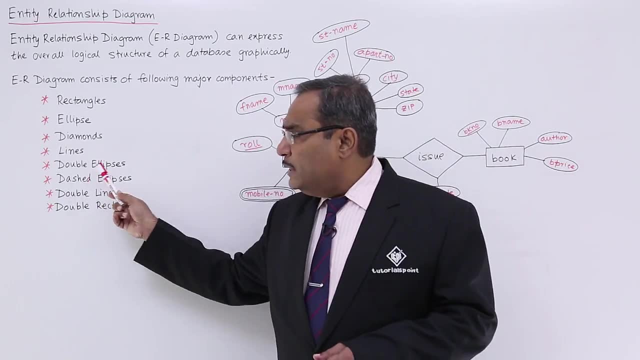 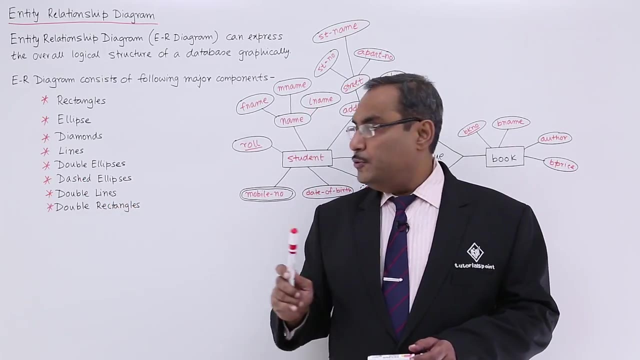 Lines will be denoting the links between, say, attribute and entity. entity and relationship Links will be denoted by lines. Double ellipse will be denoting the multivariate attribute. Dash ellipse will be denoting the derived attribute. Double lines will be denoting: 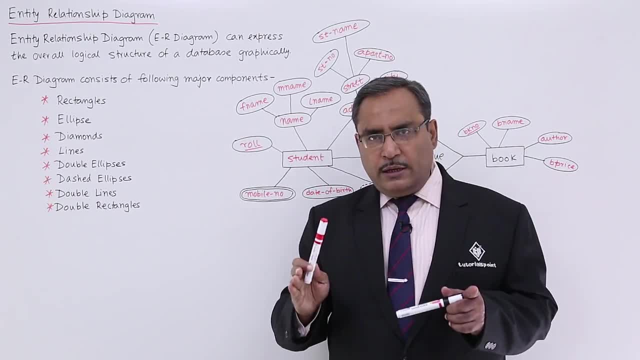 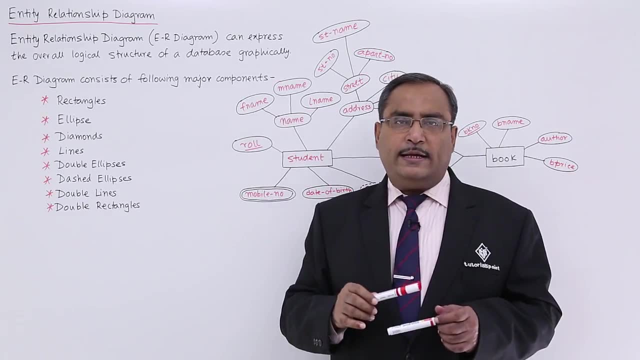 total participation that is merging in between the relationship and the entity, And double rectangles will be denoting the weak entity set. So weak entity set means that entity set which does not have any primary key but can have partial key, So that entity will 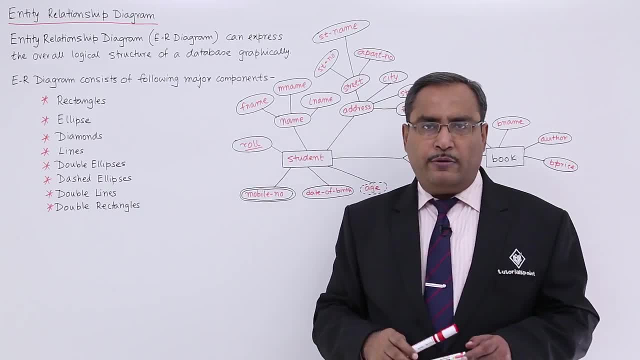 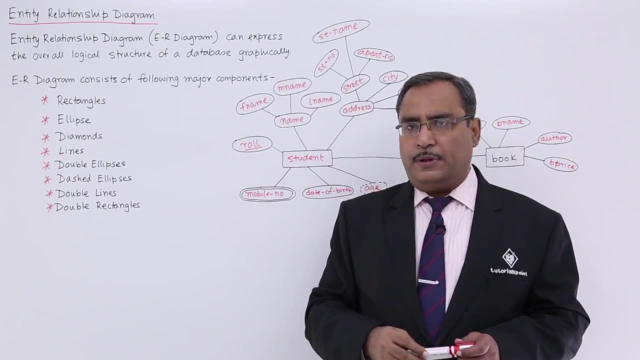 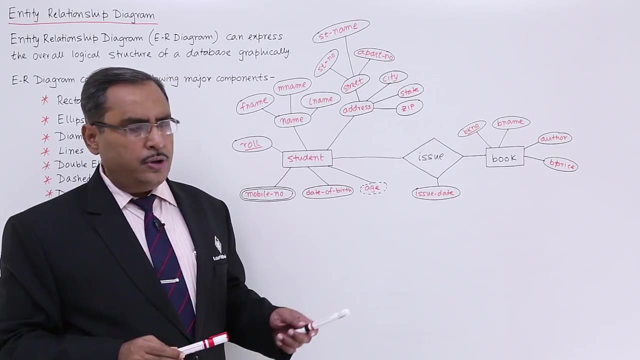 be known as the double rectangles, will be denoted by the double rectangles in the entity relationship diagram. i think our conception will get clear if you go through one example here, you see this is a very simple example which we discussed in our earlier videos also. so here the student is one entity, here this book is another entity. as a result of that, 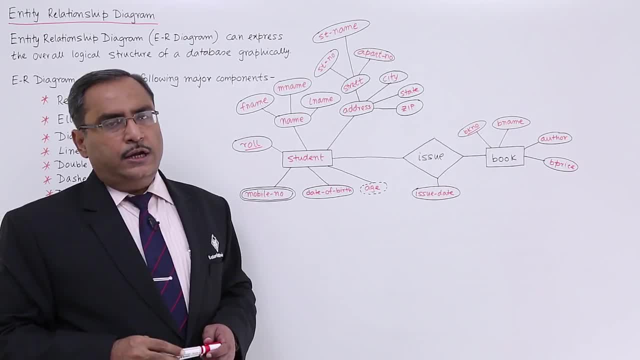 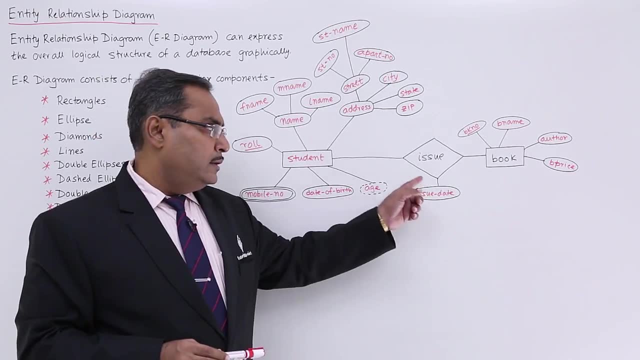 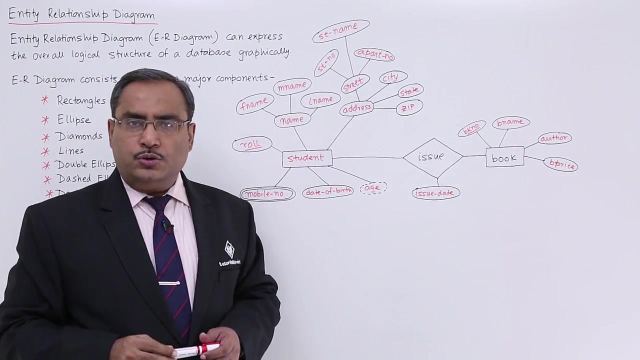 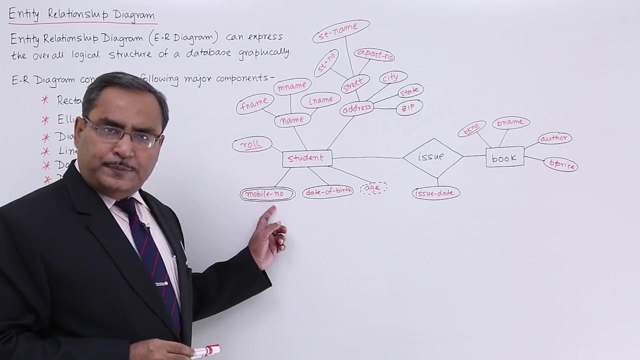 this student and this book. they have been kept in rectangular boxes. so this is my issue. issue has been put within a daemon box denoting the relationship, and all these attributes are enclosed within ellipse, denoting that they are attributes. this double ellipse will be denoting the mobile number, which is a multi valued attribute. 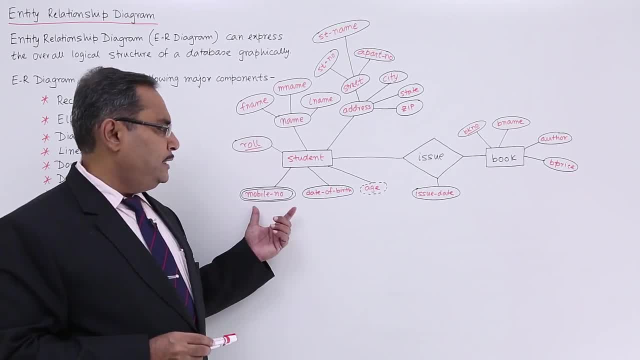 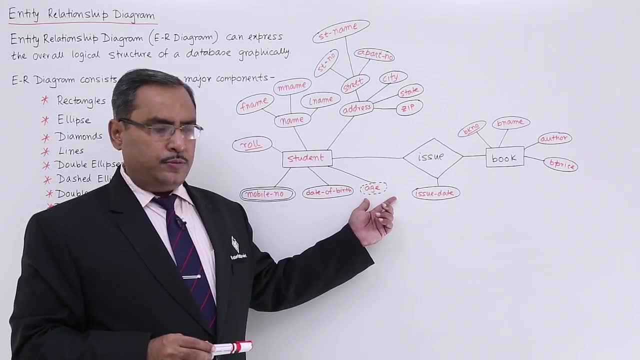 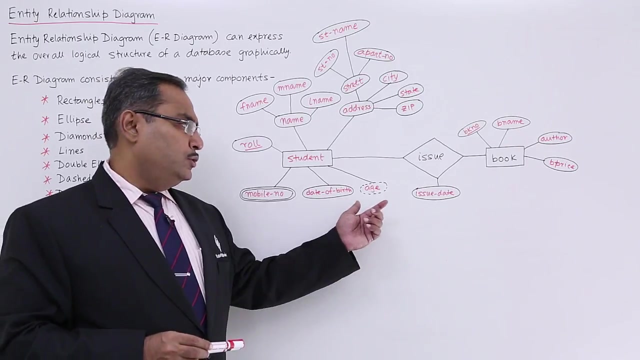 that is why A student can have multiple mobile numbers. so that is why it is multi-valued attribute and put within double ellipse. This dotted ellipse is denoting the derived attribute, because if you know the date of birth from the system's current date, we can easily calculate the age of a student. 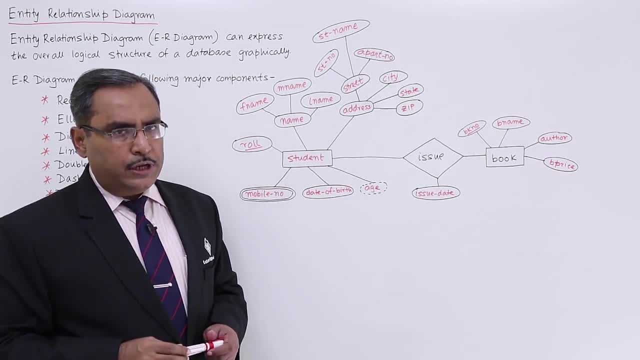 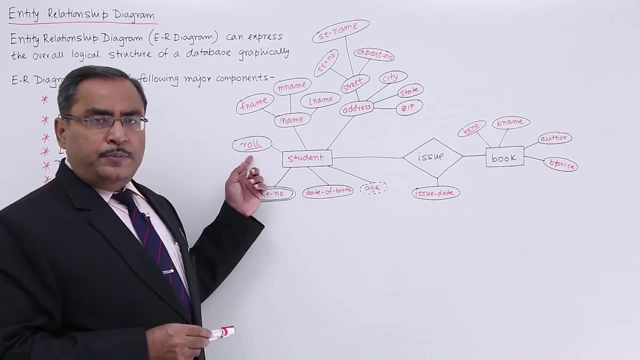 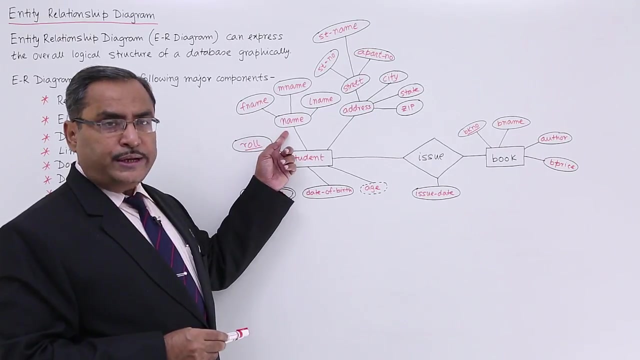 So this age value can easily be calculated using some calculations or business rules or something. So those attributes will be known as the derived attributes. This is my prime attribute, so that is why role has been put underlined. This is my name. is there, which is a composite attribute, has been decomposed into the simple. 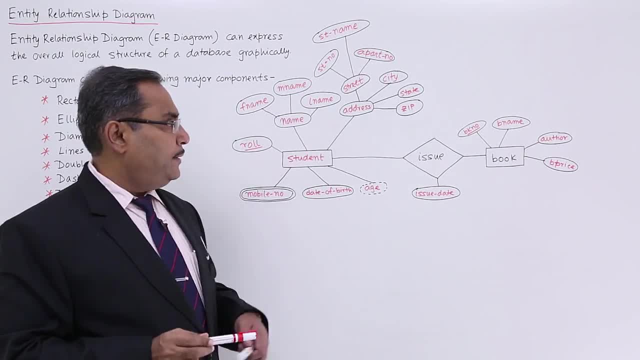 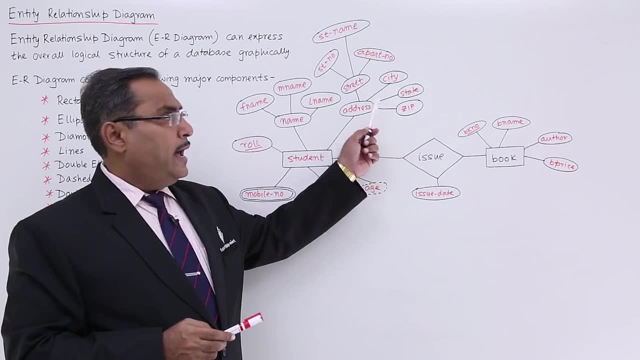 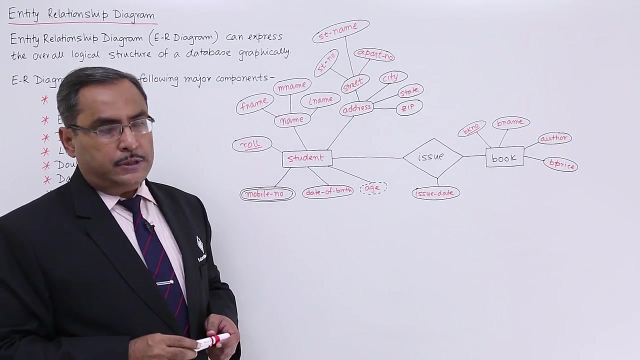 attributes: first name, middle name and the last name. Address is also a composite attribute consisting of three simple attributes: city, state and zip, And another composite attribute is street, so street is having the street number, street name and apartment number. 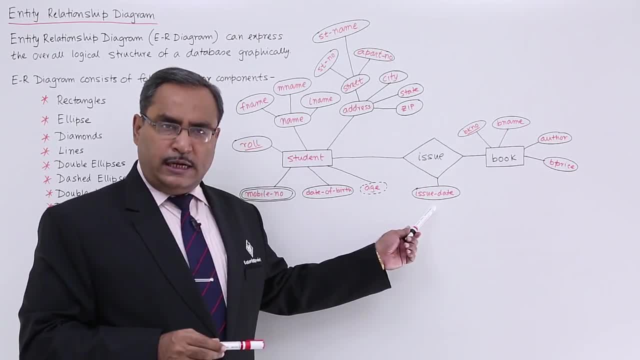 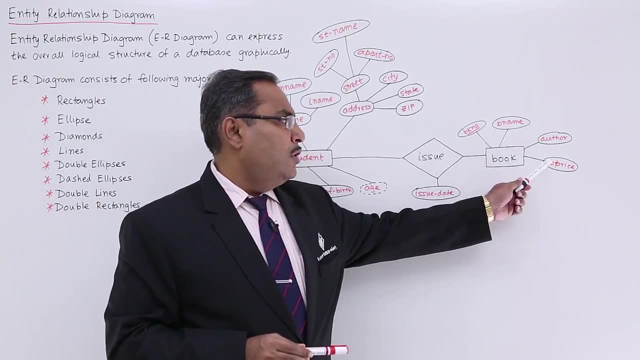 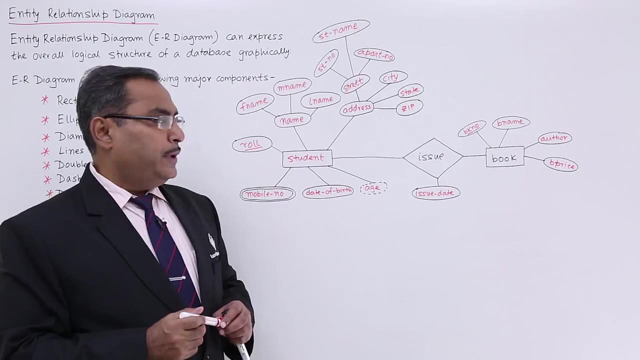 So this is my issue. Issue is having one descriptive attribute that is issue date and this is our book. that is another entity and which is having three non-prime attributes and one prime attribute. Here the prime attribute is book number. So in this way we can have say, this book can have, say, another attribute. 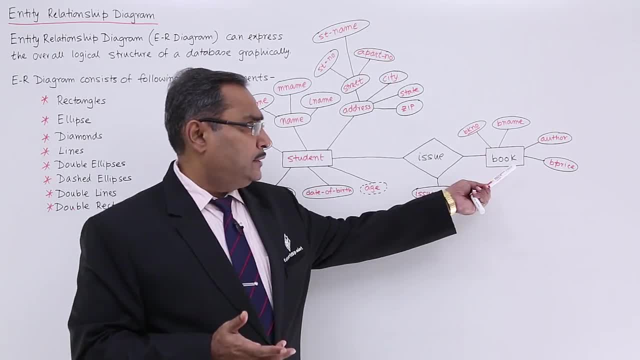 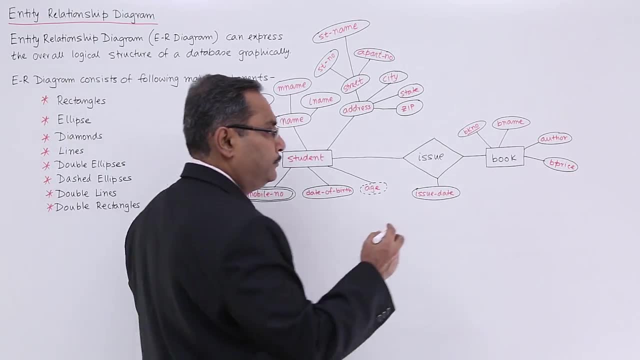 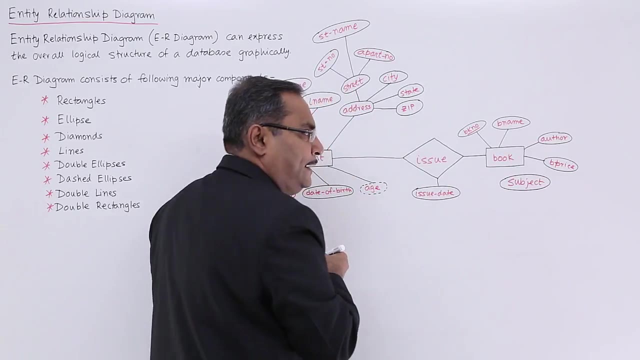 Let it be say subject. let it be subject because in our previous example we had one attribute linked with the book, So let me put that one. So this is my subject, which has been put, and it will be related with the book entity. 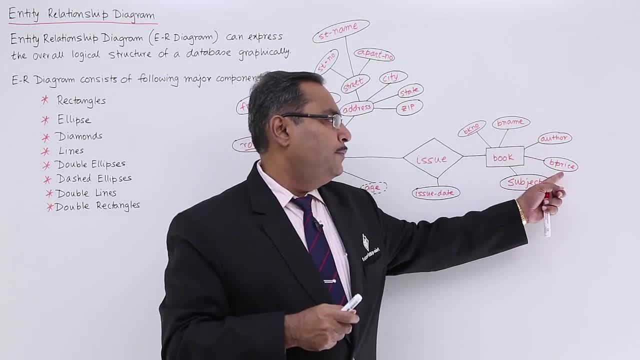 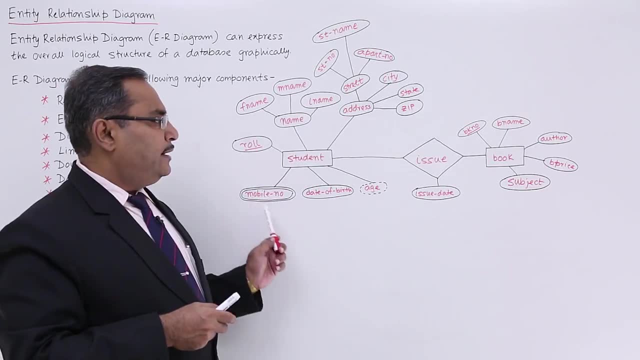 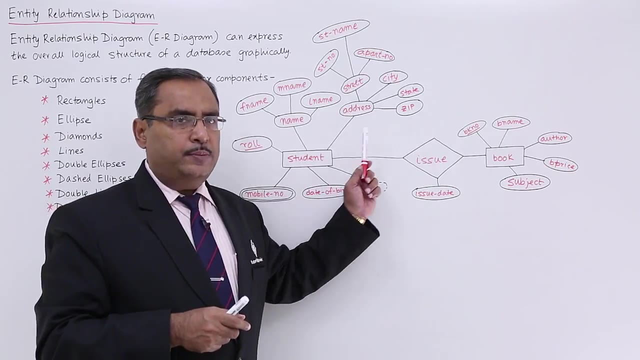 So here we are having this book number, book name, author, book price and the subject of the book, And this book number is the prime attribute. So in this way, you see, there is a graphical representation of this particular library management system consisting two entities: student and book. one relationship issue. 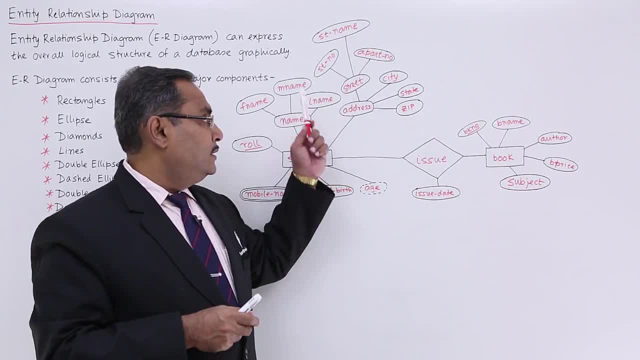 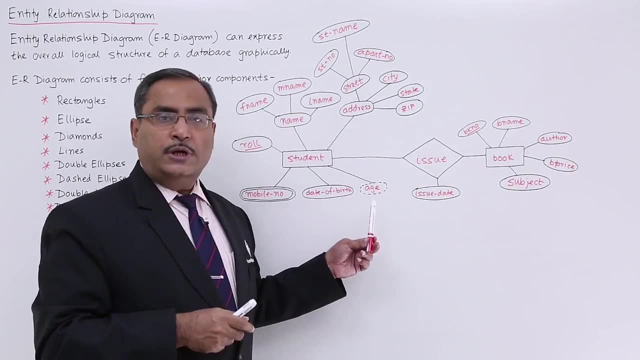 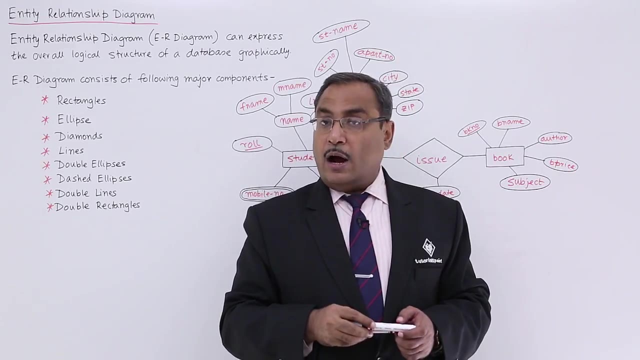 one descriptive attribute, that is, issue date, and other attributes are there. Some of them are multi-valued, some of them are composite, some of them are simple attributes and some of them are derived attributes. So in this way, we have discussed what is year diagram and how to draw them. 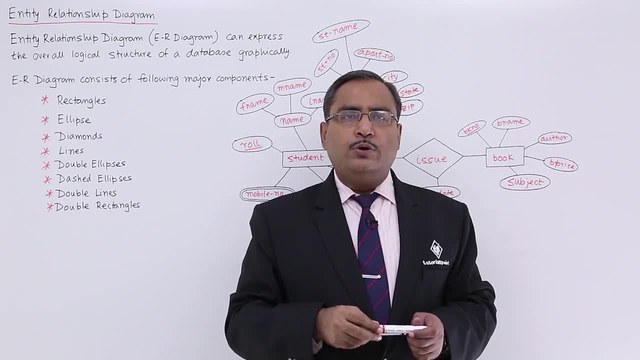 In the next video we shall discuss multiple different symbols which we will be using in our year diagram. Please watch that video also, and thanks for watching this one.